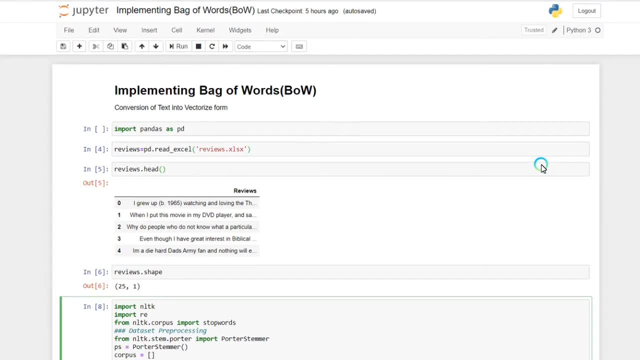 hello everyone. in this particular session I am going to implement bag of words in Python. so bag of words is basically the conversion of text into some vectorized form, as I have already mentioned in my previous session. so for that, what I'm doing is I am first importing the pandas library to reading. 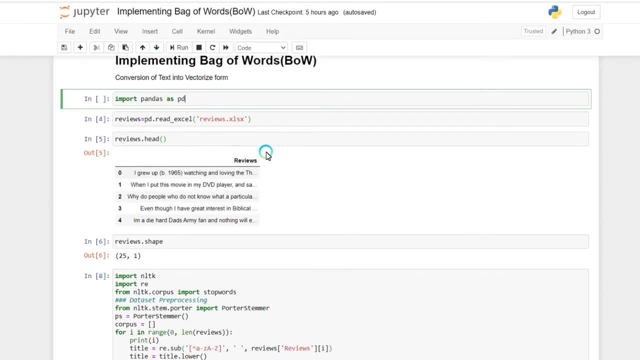 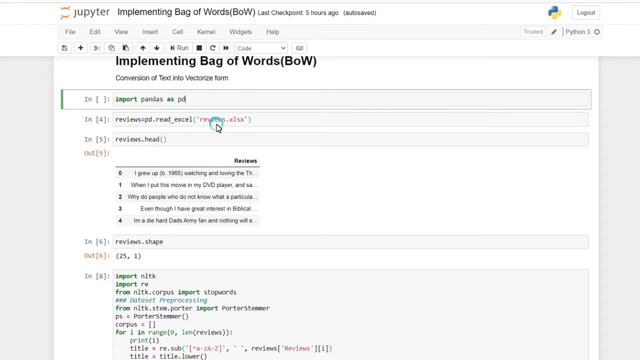 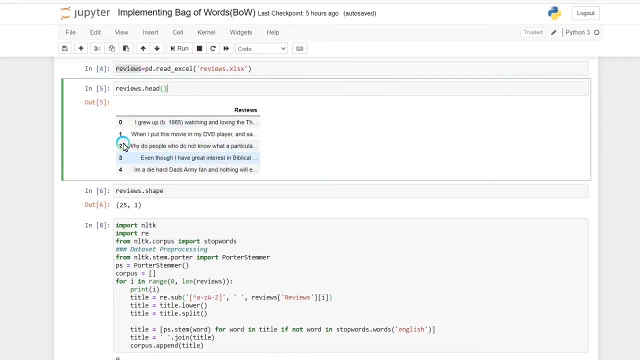 my to read my data set. so here I am using the data set of movie reviews, which contains around 25 rows for 25 postments or 25 movie reviews. so first I'm reading my data set into the reviews variables, so operating just playing the first five rows of my data set so I can see here, like the: 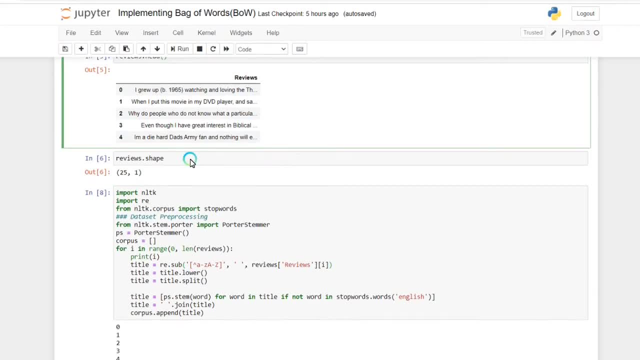 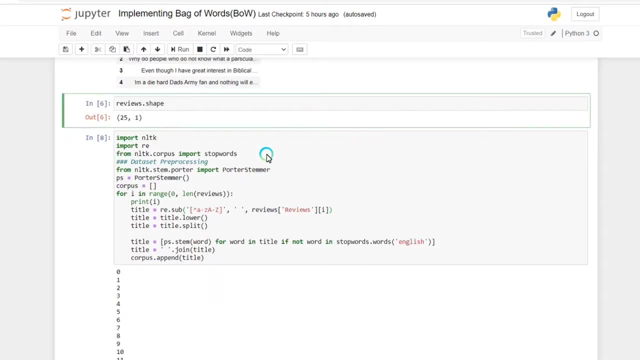 different initial reviews are present here, right, so here the same of the reviews, that is my data sets. so it contains around 25 reviews and one column. so now what I'm doing is I'm doing some pre-processing of to remind the set. so for that, what I'm using is an NLP key and regular expectation library. 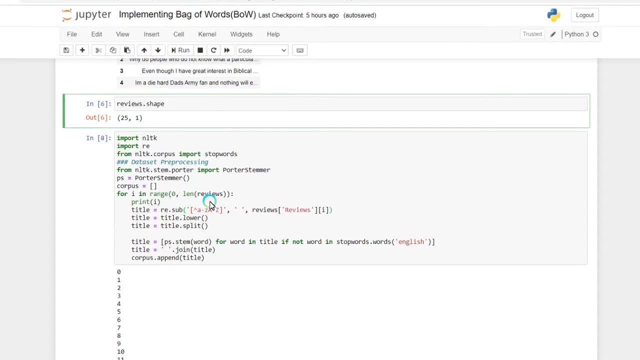 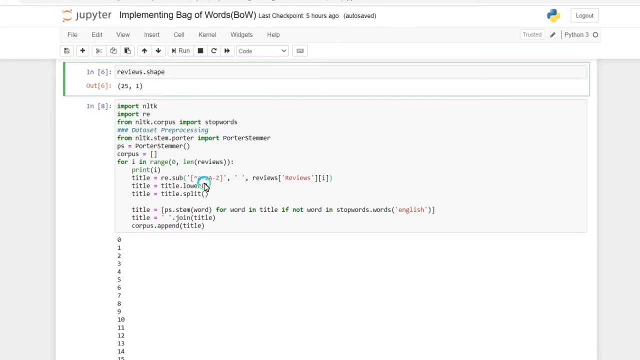 so Here what I'm doing is I'm executing a for loop from the first sentence to the last sentence of my dataset. So here this is the for loop and here I'm removing the special symbols or different numbers that are present in my dataset or present in my reviews. 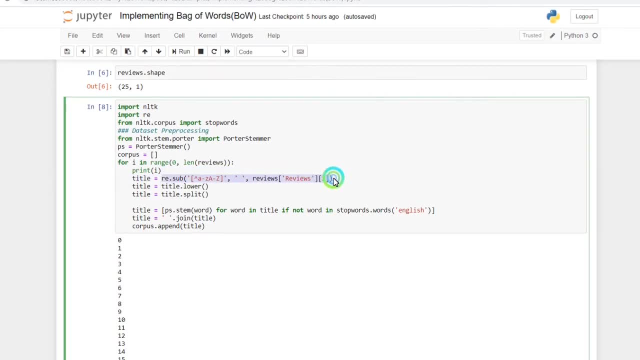 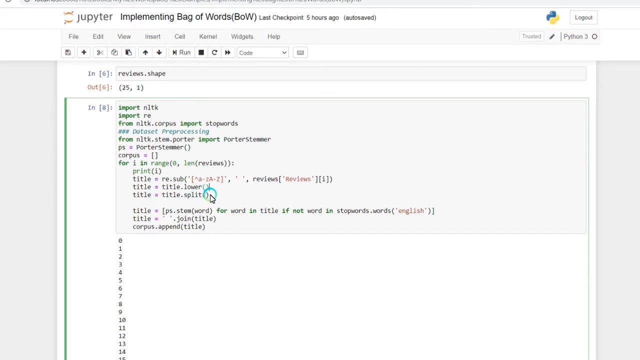 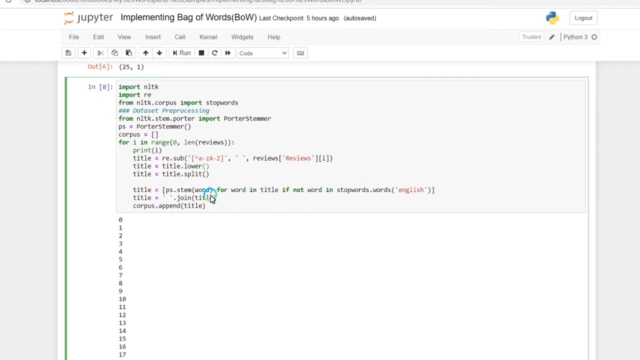 So this particular expression is removing all the special symbols and numbers from my reviews. So, after removing, what I'm doing is I'm just converting all the reviews into some smaller lower cases, that is the lower case. So after converting the lower case, I'm splitting every single words from the sentence. from every sentence I'm removing, splitting all the words and after removing, I'm checking, like, whether this particular word is stop words or not. 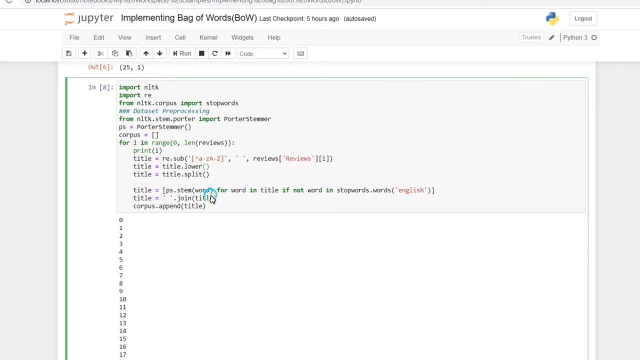 Like, if it is a stop words, I'm just removing all the words from the sentence, removing that word, and if it is not a stop word, i'm keeping that word. so stop words are basically the words which are less important to my, to my data set. so suppose we can. for example, you can say: 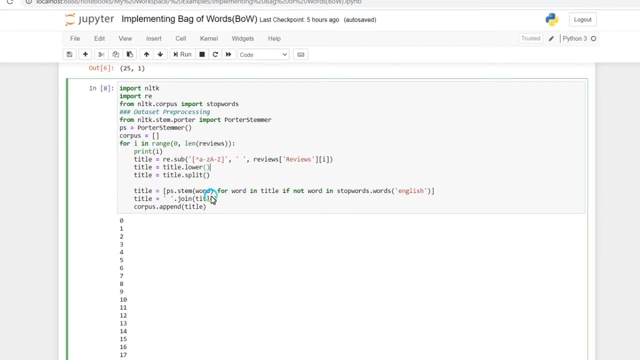 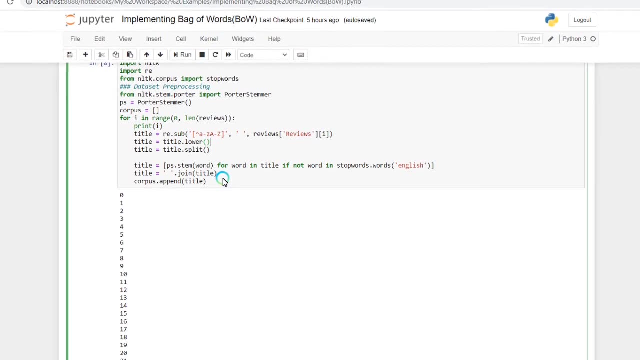 he is. and these are some stop words which are less important to my data set. so, after removing the stop words, i am again joining my words into the title. so, after joining, finally adding all the titles to my corpus. so finally, after executing this command, i can see my corpus is here, so it 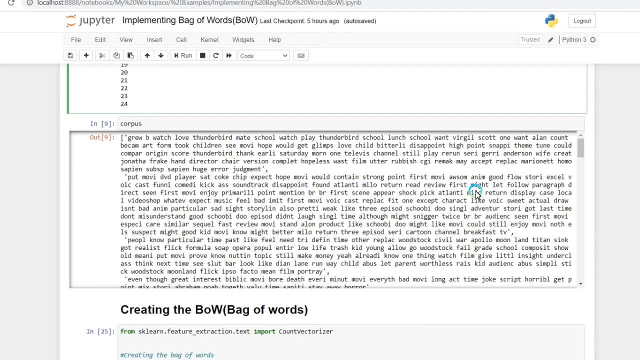 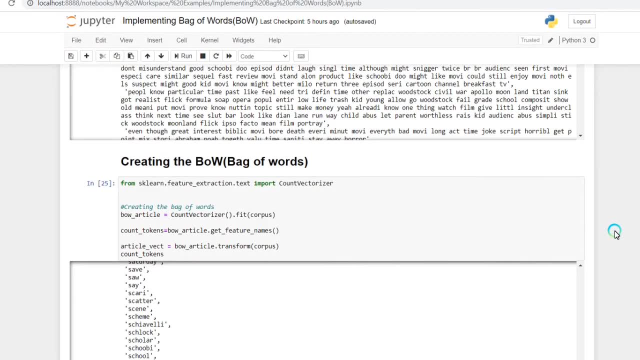 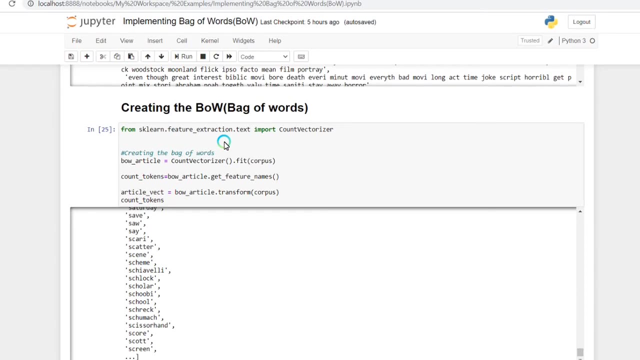 contains all the movie reviews in some proper format. so finally i got my corpus here and now i have to convert this corpus into the bag of words. that means the counter vector. so here i'm doing is i'm importing the counter vector from the sklearn library. so after importing 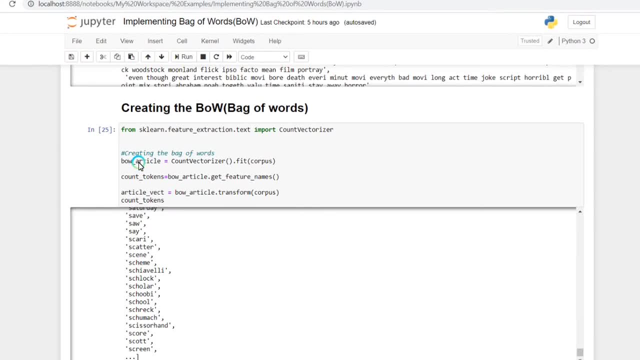 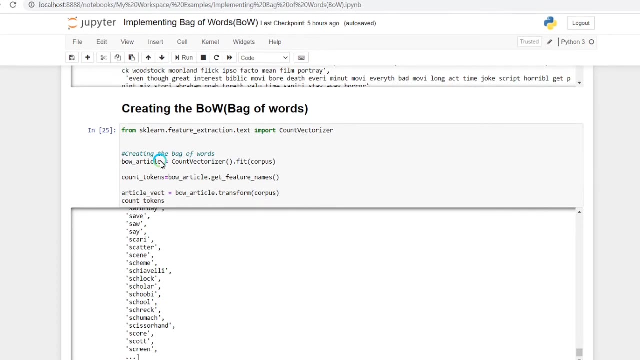 the counter vector, i'm creating my bag of words article, like big of words, um variable. so i have given to my even my corpus to the bag of words, like the counter vector and after giving it converts all the sentences into that vectorized form, and also i'm extracting all the features by using this particular command, like all the 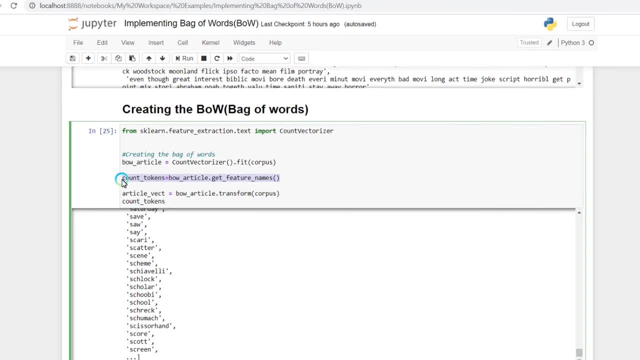 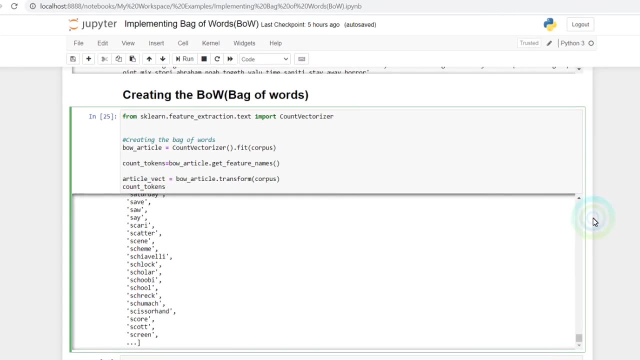 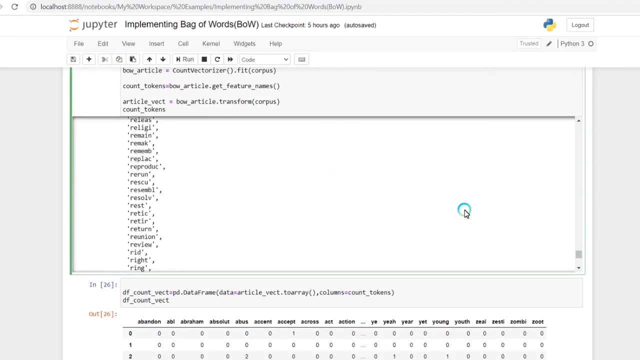 features of my data set, that is, all the words that are present in my data set. so, finally, i am transforming my corpus into the vectorized form and here i am displaying all the features. that are all the words present in my data set. so after extract, uh, displaying the data set, i can see here: 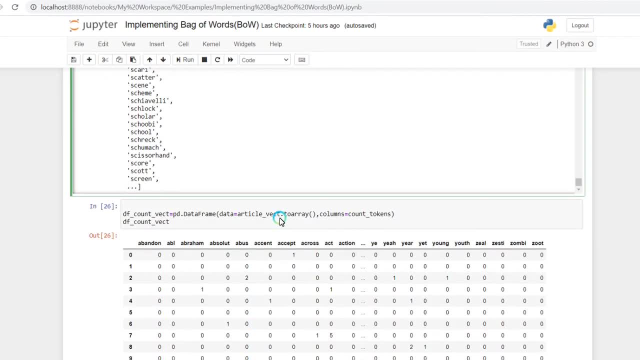 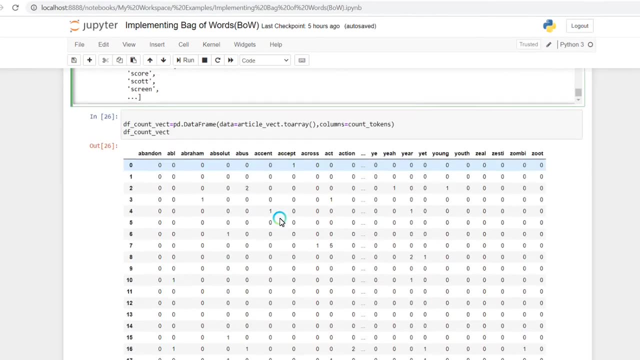 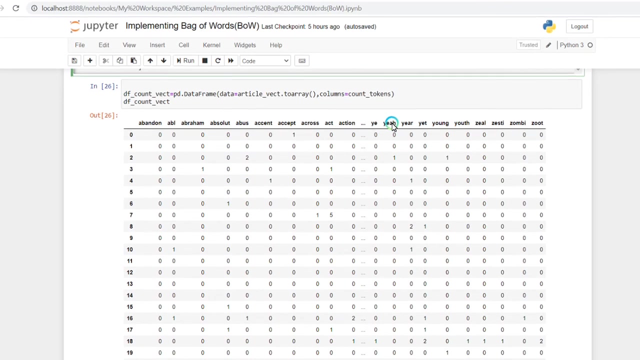 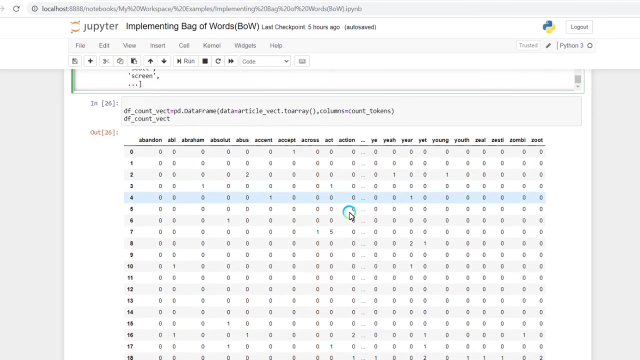 the words are present here. so, after that, here, finally, i am displaying the factor that is formed using that counter vectorization vectorizer library. so this is the vector, the complete factor, where you can see different words are there which are in the uh, which are considering as features for my data set. so, and total 25 rows are there, that are, 25 sentences are there. 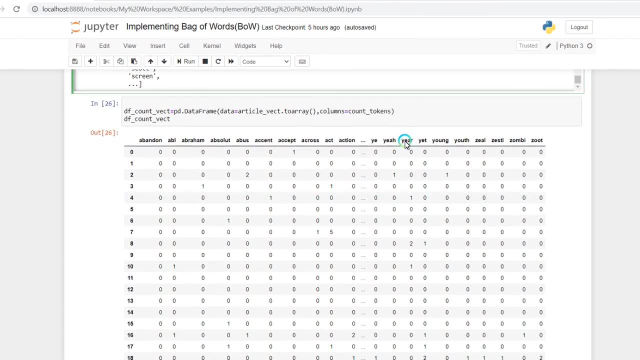 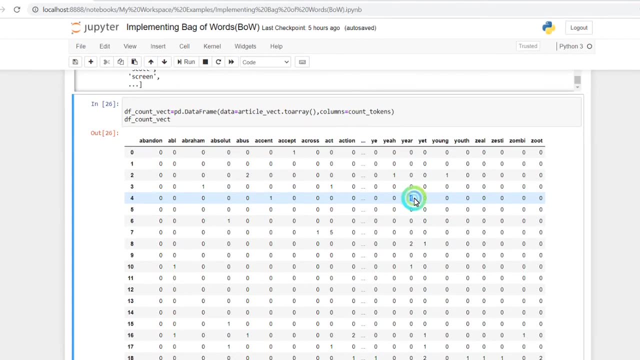 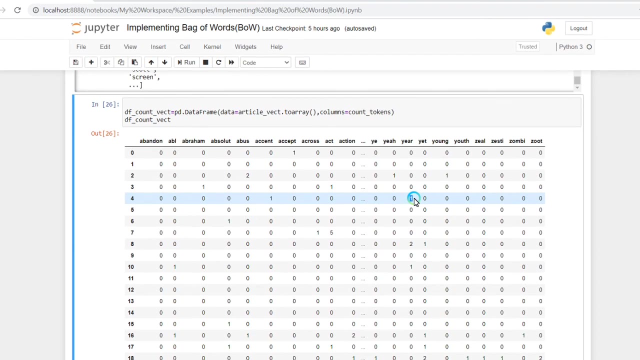 so here you can see: if a particular year, suppose particular word- suppose here is here- is present in the fourth sentence, so it's assigned one there. so if your word is present in a particular sentence, it's assigning one there, or if it is not present, then it's assigning zero.